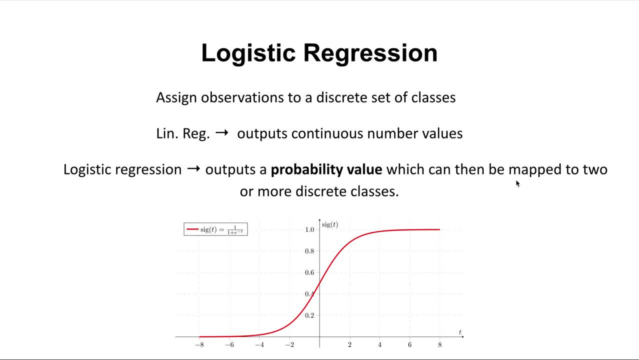 or more discrete classes. Remember, when I say discrete classes I mean something very definite, right, Discrete classes are categorical. This falls under classification. So when you think about it in the long term, logistic regression is really just a classification technique that uses a probability value to sort between two or more classes, And that's. 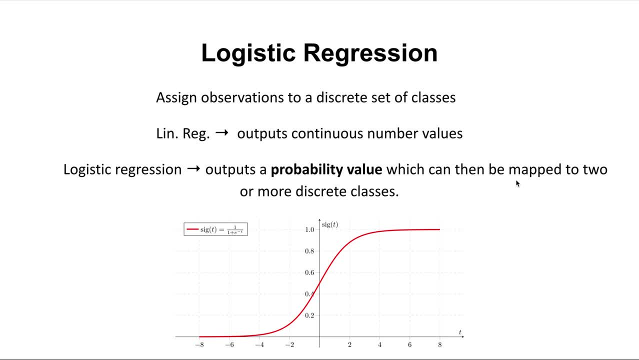 what the sigma function is doing. The sigma function provides us the probability value to one of those discrete classes, And I guess people confuse this with linear regression because the name is logistic regression, right, But the idea is that it's logistic because it makes use of a logistic function. 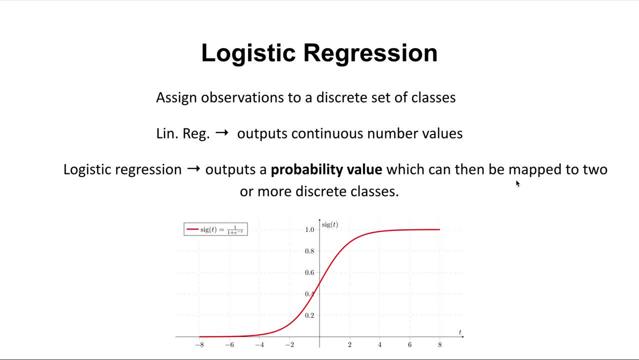 like the sigmoid curve right which is seen in this slide, And remember the broad idea here, or the broad intuition behind this, is that logistic regression uses probability values from the sigmoid function to assign observations to a discrete set of classes. That's what logistic regression is really just doing. 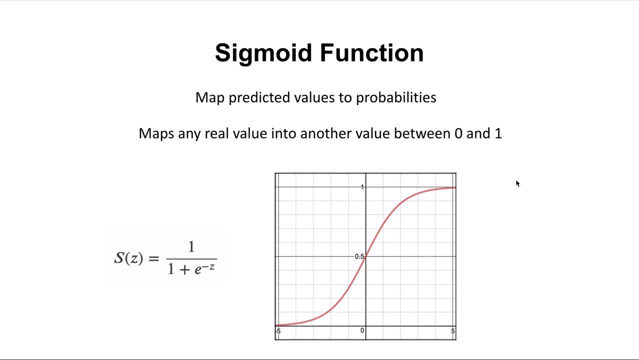 Let's move on. So let's talk a little bit more about the sigmoid function. So the sigmoid function is the function that helps us map predicted values to probabilities right. So the sigmoid function is that equation 1 over 1 plus e to the negative z, And this equation basically just denotes: 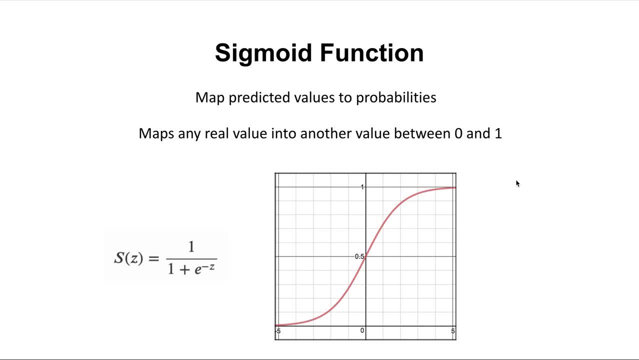 the output for a certain probability function, right input-output. And what's going on with the sigmoid function is that we're taking our input and we're mapping it to any real value between 0 and 1. And that's really impressive. 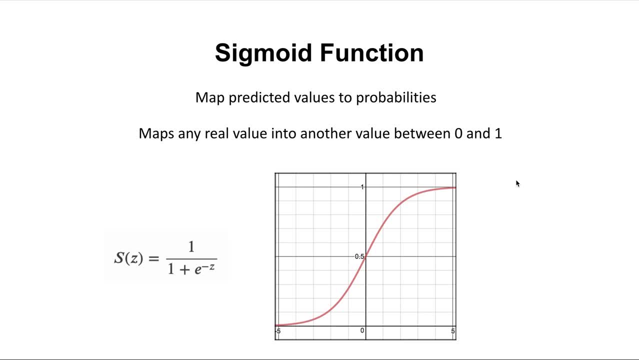 Because when you think about it, you're getting a distinct real probability value between 0 and 1.. And then we can think about that probability value and determine whether it's a certain class or a certain different class. At the end of the day, this probability value 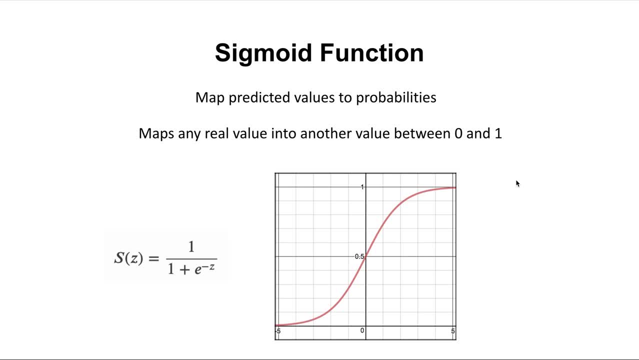 that's spit out by the sigmoid function. this is not the main thing that we want from logistic regression. This is just one step in the process of logistic regression, because in the long run, logistic regression is a classifier, like I said earlier, And with classifiers. 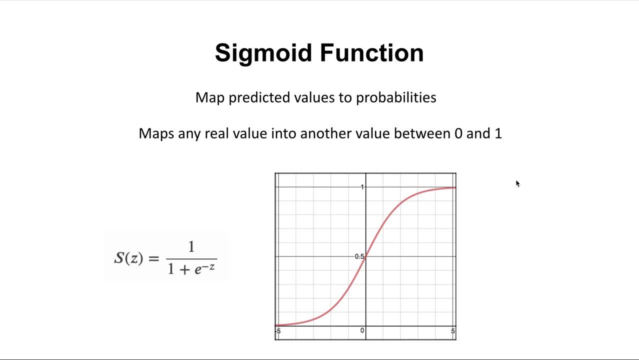 we want a discrete output, And remember, by discrete I mean categorical. So this isn't really categorical, right? This is just a continuous probability value. So what we want to get out of this is we want to turn this probability value from the sigmoid function into a discrete, class-valued output. 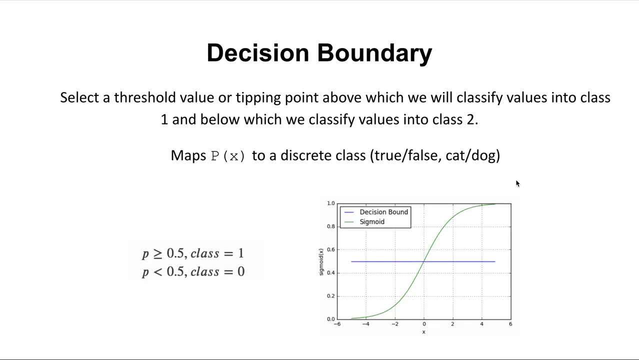 And I guess we're going to find out how to do that. A decision boundary is how we do that right. So a decision boundary is really just a threshold or really a line of separation. That's basically when we select a threshold value or tipping point above which we classify. 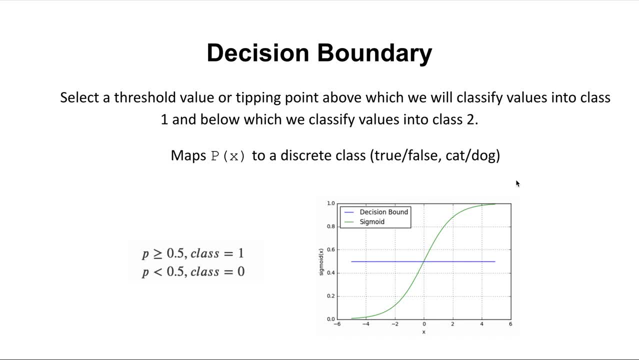 values into class 1. And below which we classify into class 2.. This is really important, because this is where we basically separate between our different probabilities, right? So take a look at this graph that I've given on this slide. In this graph, it's a sigmoid. 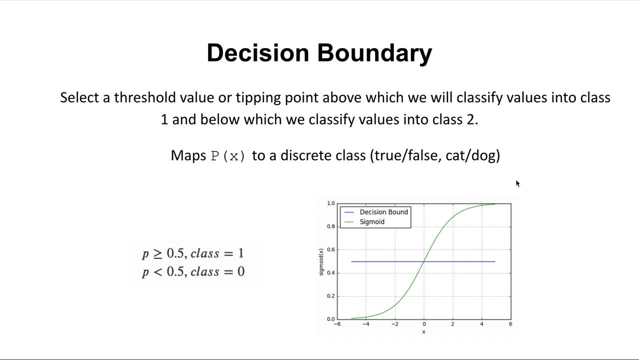 function and there's a decision boundary at approximately 0.5.. This decision boundary is basically saying that any probability value, any p of x above 0.5, any continuous probability value above 0.5 can be considered a certain discrete class, like cat or dog, for example. 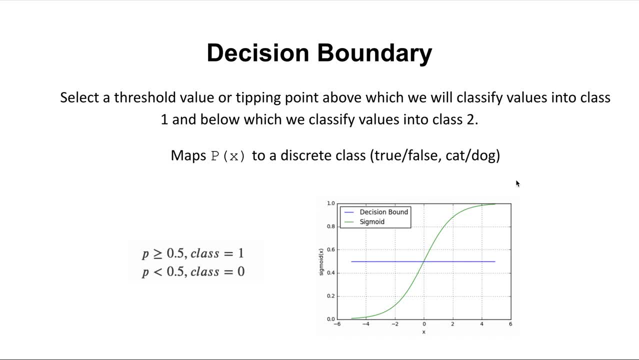 cat And any probability value below 0.5 or any p of x probability function value below 0.5 can be modeled. vice versa, the other class. So what's going on here is that the decision boundary acts like a function that separates. 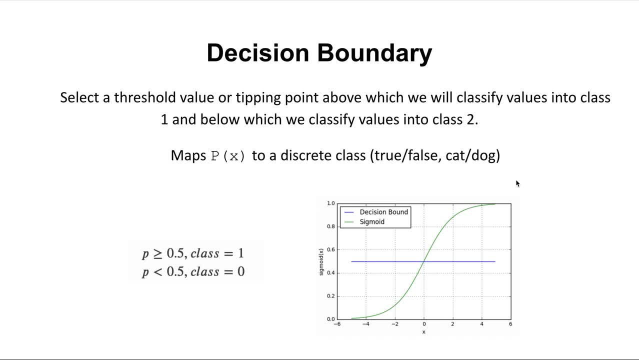 between the probabilities and helps us to map to discrete classes. Without a decision boundary, logistic regression is useless as a classifier because we don't want a probability output right. The probability output is useful, but it's only useful to a certain extent, because we 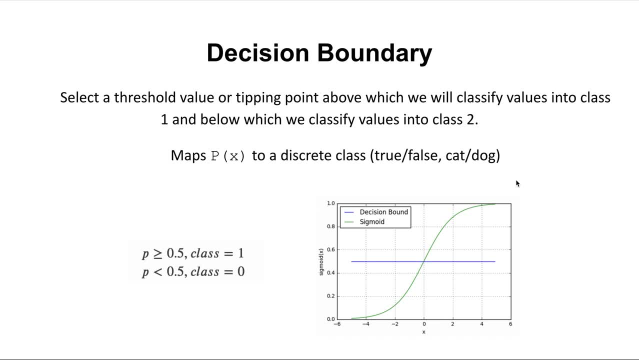 want that final classification output. We want to know the category right. If you're predicting cats versus dogs, knowing the probability of an image being a cat or dog is definitely useful information, but it's not ideal because we want to know. can. 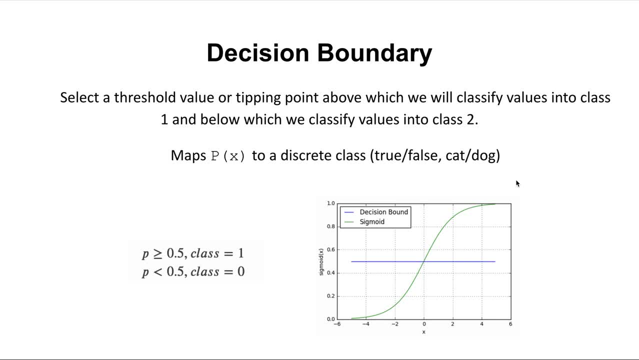 you predict it as either a cat or dog- definitively- And a decision boundary allows us to do that because we get a definitive answer for whether our probability is above or below the decision boundary, And for more complex, sigmoid curves and more complex functions of interest for logistic. 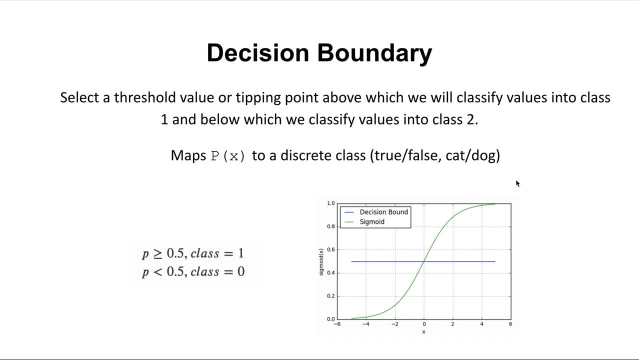 regression, the decision boundaries get more complicated. right, It's not just always a simple, pretty horizontal line. The broad idea here is that for a decision boundary it's important, because it's basically what's so special about logistic regression: It helps us define between two different classes. 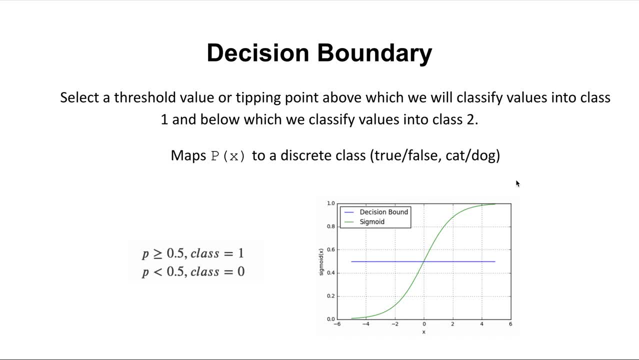 And, as you can see on the left side of this slide, you can see that this is the actual functional notation for this decision boundary. So you see that if probability is greater than 0.5, the class is equal to 1.. Probability is less than 0.5, the class is equal to 0.. 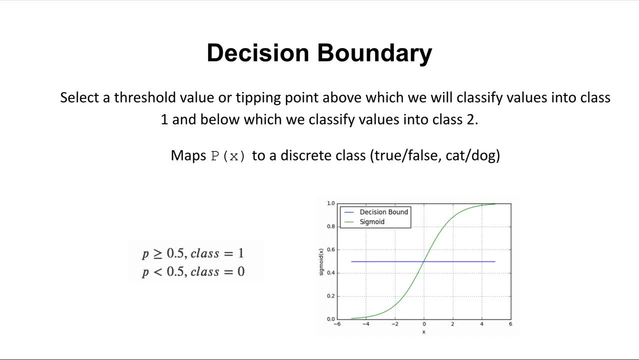 It's relatively simple mathematics right. The decision boundary is what divides between the different probabilities and allows us to classify whether a certain probability value, p, is a certain class or a different certain class. So that's what's going on with decision boundaries. 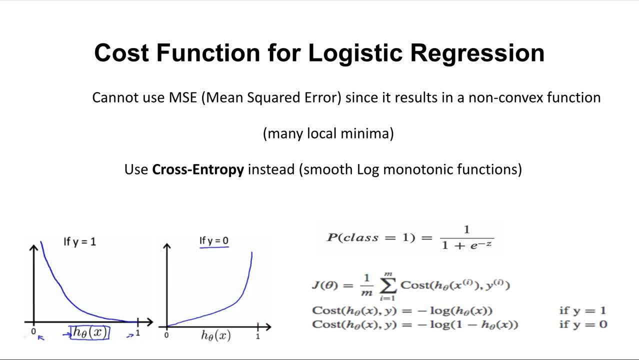 Let's talk about the cost function for logistic regression. So for linear regression, the cost function is mean squared error right, And we cannot use mean squared error in this case because it results in a non-convex function for logistic regression. Why is a non-convex function bad in this scenario? 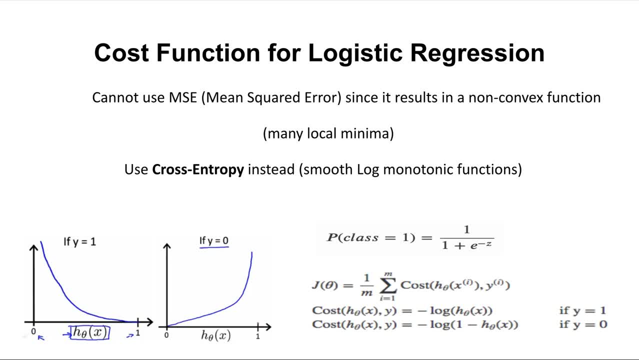 A non-convex function has too many local minima right. So what's the point of doing a loss minima, A loss minimization, on a function with many local minima right? We want a function with one absolute local minima. 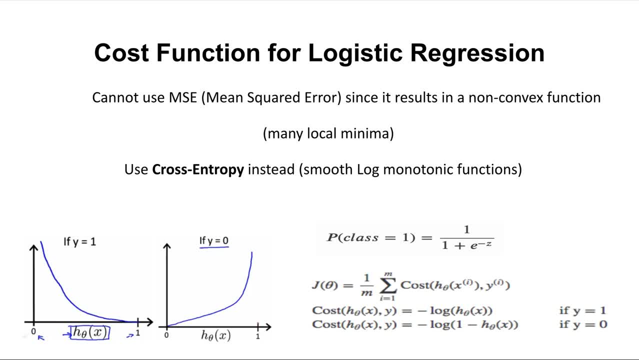 One point where we can definitively say: oh, we found the minimal loss point. So for logistic regression, the cost function is instead this time cross entropy. Why is it cross entropy? The cross entropy function is really just. you can think of it as a smooth logarithmic. 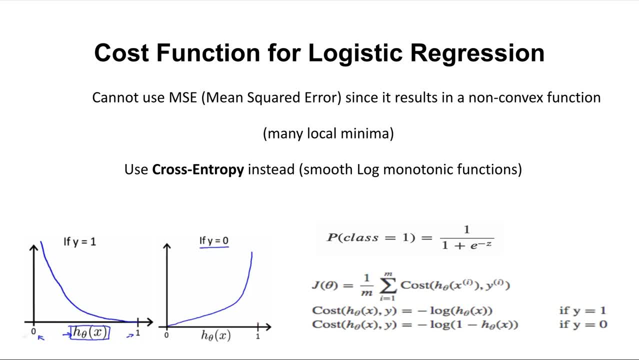 monotonic function right. It's relatively simple. The slide on the left is taken from Andrew Ng's machine learning slides and it really well illustrates the idea of the cross entropy curve. It's a really simple, downward sloping logarithmic monotonic function. 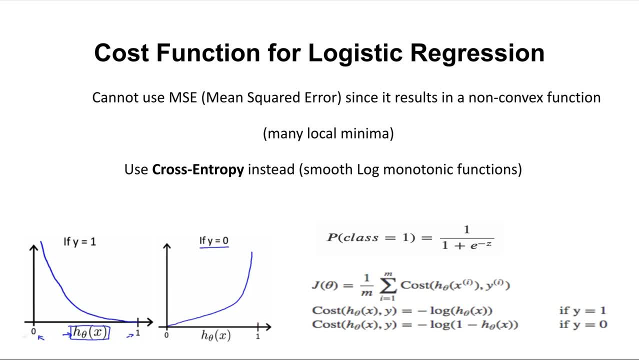 And, as you can see, it's really easy to identify where loss is minimized, right at the point where it's lowest. And that's really important because there's not that many local minima. There's one absolute minima, And that's why, for the case of logistic regression, cost entropy works as the best cost function. 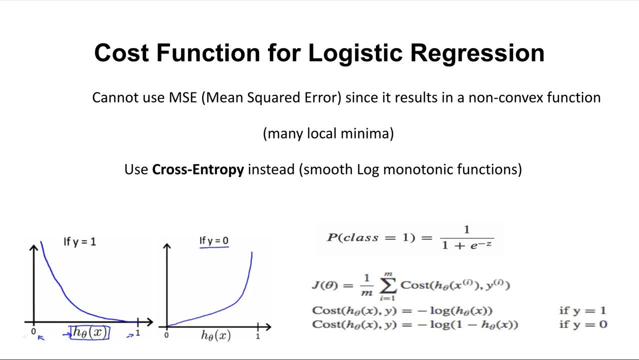 in this scenario because it doesn't result in a non-convex function with many local minima. Instead, it gives us one consolidated function with one absolute minima. So on the right You're probably thinking about this. On this slide you see some of the actual algebraic notation for these logarithmic functions. 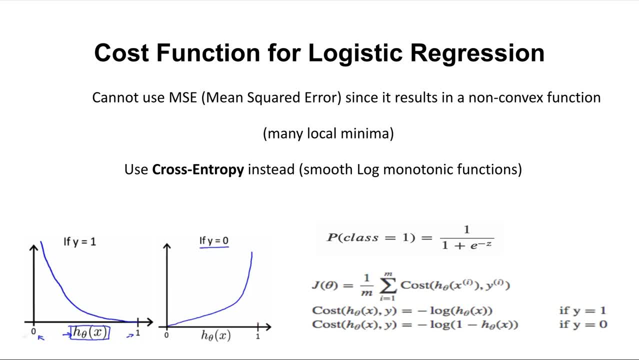 for cross entropy. You don't have to know this, because this is definitely out of the bounds of this course, But what's going on here is that you're just separating this into two functions, right? You're separating into it if we're deciding on class one, if y equals one, if we're deciding. 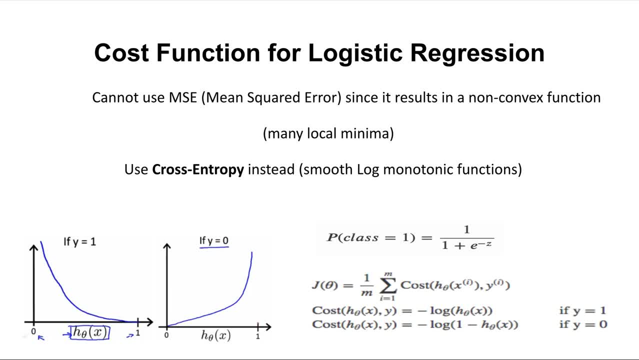 on class two, if y equals zero, And then for both of those you have separate cost functions, right, And both of them are smooth, logarithmic, monotonic functions, And so the main intuition I want you to understand here is that we don't use mean squared error. 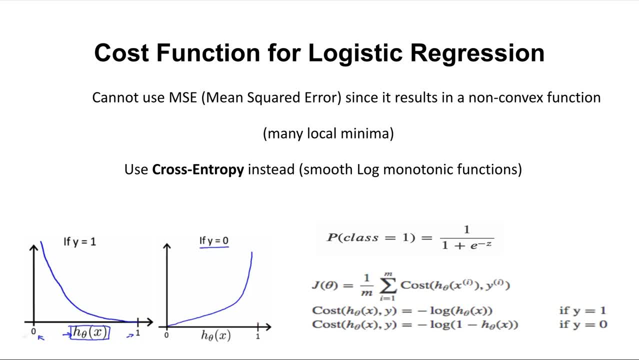 We use cost entropy because it results in a convex function with only one local or absolute minima, And that's why it's important to use cost entropy in this case. Let's move on. Let's talk about a practical example of your logistic regression action. 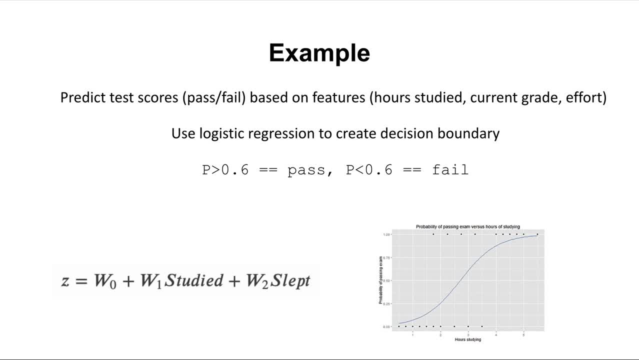 So let's just have an example where we're given data on the time spent studying and exam scores, right We end. So the idea is that we want to predict test scores- pass or fail- based on these features right, Like the time studied, the exam scores, the current grade effort, et cetera. 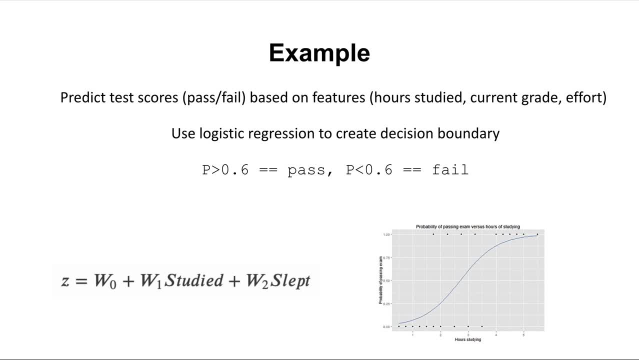 And what we can do is that we can use logistic regression to create a decision boundary, And so this is what our decision boundary would basically look like. in a really simplified scenario, It would be that if the probability of the student doing well is greater than 0.6, they 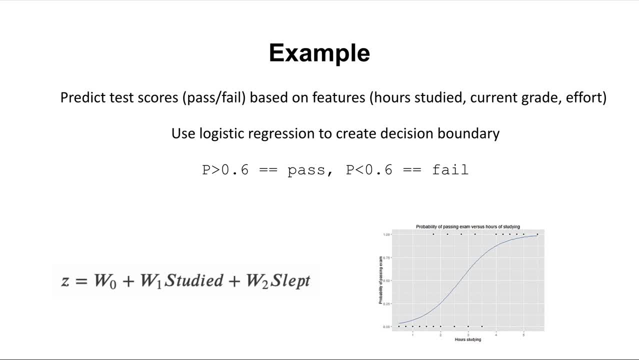 most likely passed right. We can discreetly assess them as having passed. If the probability is less than 0.6, they most likely passed. If the probability is less than 0.6, they most likely failed, And then we can assess that as a discrete category of having failed. 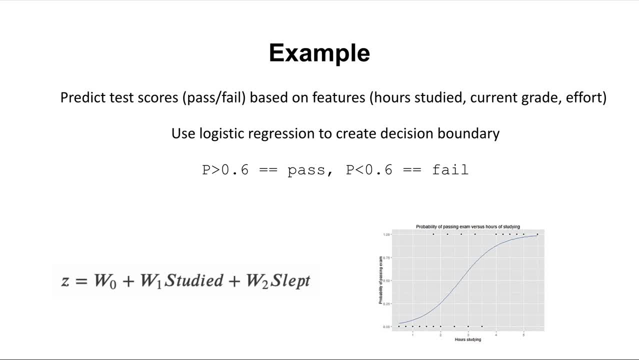 And so we can model that in that graph that you see below, where we can place a decision boundary at any arbitrary point, as long as it makes sense. And on the left you see how this equation would be kind of modeled, right. 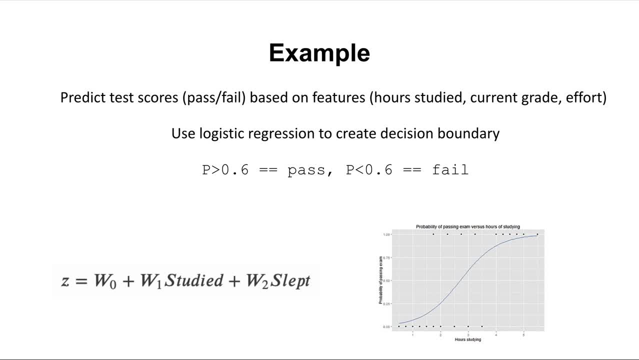 For a linear decision boundary And the idea is that, regardless of what the problem is, you always do the same thing with logistic regression. right, You have your sigmoid function or some kind of sigmoid curve. You denote a certain decision boundary where you separate between the different probabilities. 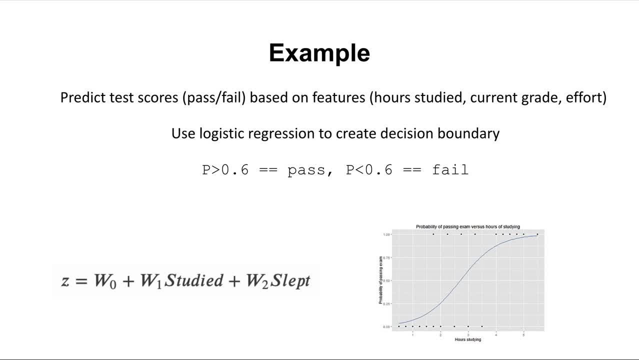 And then you do the same thing with logistic regression And then you basically just generate data for that problem and you assess different data points on that decision boundary. And this is what the fundamental part of logistic regression is. right, It really is just the same immutable process across all types of problems. 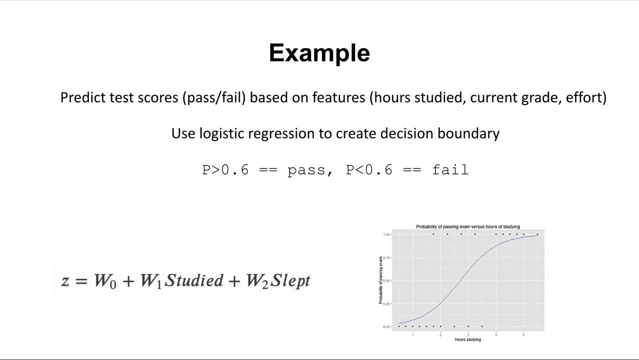 And compared to linear regression, where we're basically outputting a continuous linear numerical value, here we're outputting a probability which then gets transformed into a certain discrete category based on the decision boundary for that problem. So that's logistic regression, right. 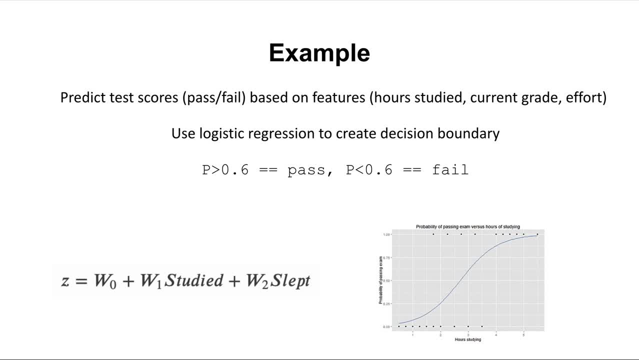 Pretty simple to understand. So people sometimes feel a little bit fazed by the idea of the sigmoid curve and some of the difficulty in understanding the cost function right. But overall it's a relatively simple principle to understand the idea of the decision boundary. 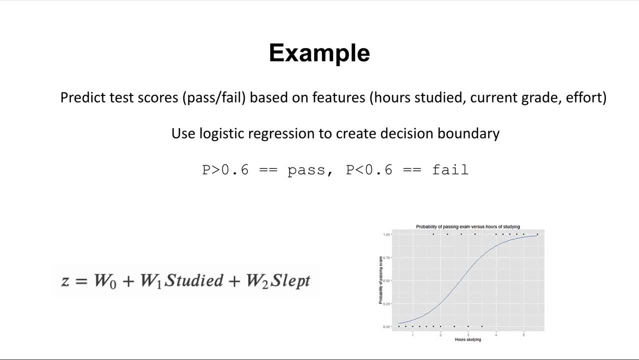 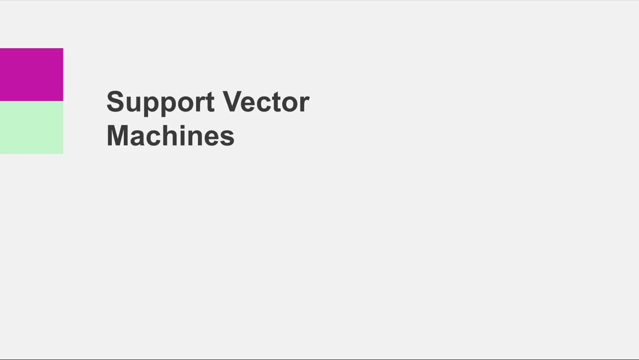 how we separate between probabilities and what's going on with how to create the decision boundary and how the sigmoid function really works as a scale of outputting probability. All right, awesome, Let's move on to support vector machines And let's kind of demystify this supposedly super difficult problem. 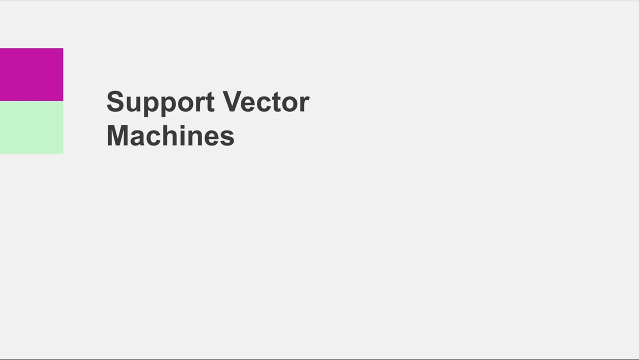 So let's move on to support vector machines And let's kind of demystify this supposedly super difficult problem. So let's move on to support vector machines. It's really like a vocab classifier point. It's basically an extension of perceptron being a similar and cręp, because each of 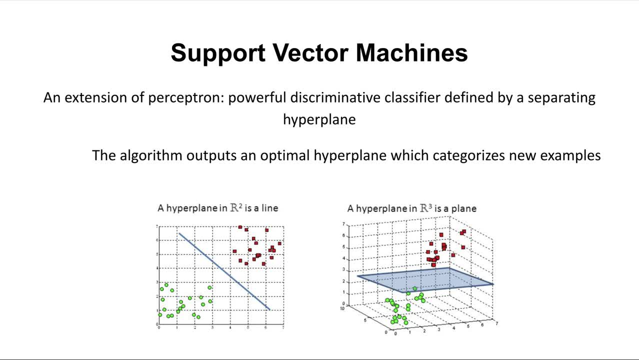 these defined by separating hyperplane. Let's reformulate that In other words, we're given some labeled training data, like any supervised learning problem, and the algorithm outputs some optimal hyperplane to categorize new examples. So what is a hyperplane? Take a look at the graph at the 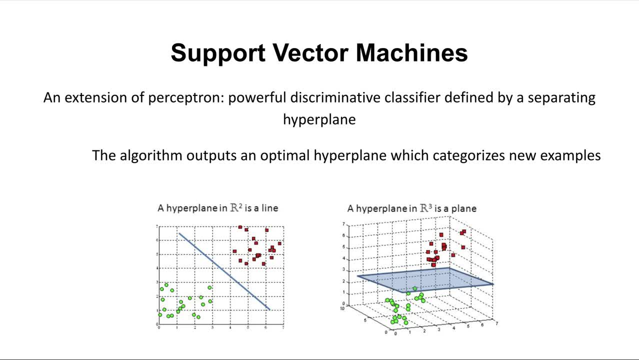 bottom of the slide on the left, and you see there's two clusters of data. This is the graph in R2, the second dimension, X and Y, And there's two data points in this graph. I'm sorry two, not two data points, two data clusters in this graph, and there's a line between them. That line between: 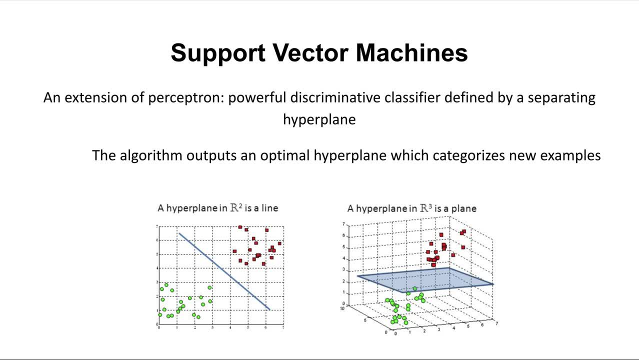 those two data clusters is known as a hyperplane. The hyperplane is the discriminative line that separates clusters or points of data or data points. So hyperplane is just another word for separating line. When you create a support vector machine, you're basically telling a classifier to 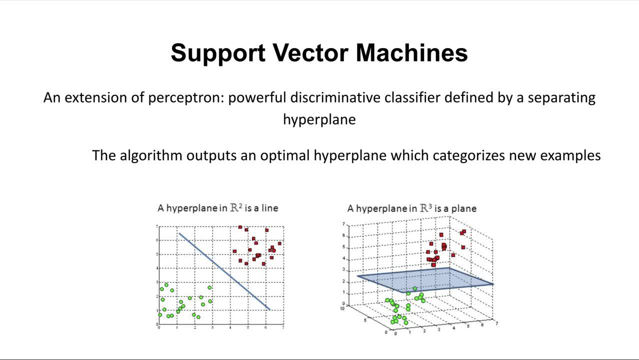 oh hey, classifier make a line that divides between some clusters of data, And this is what the algorithm does. In the end, the algorithm outputs an optimal hyperplane which categorizes new examples, And by new examples I mean we have this hyperplane in R2 for that data set. We can. 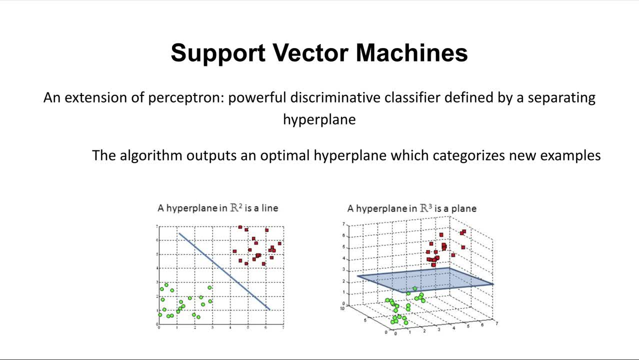 plug in a completely new example and based on the positioning of the hyperplane in that new example, we can basically say whether it falls in this category or this category, right or yellow or red. And if we want to categorize a hyperplane, we can categorize it in this category, right or 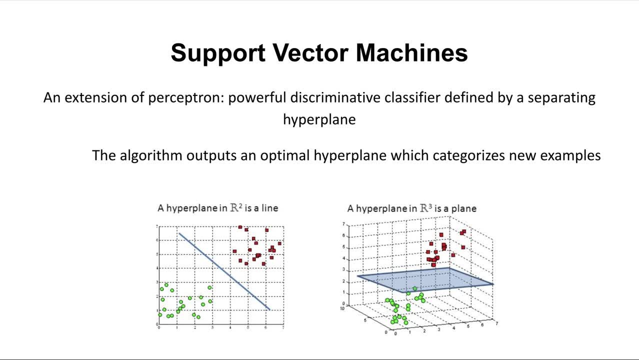 yellow or red, And if we want to categorize a hyperplane, we can categorize it in this category, right or green. So if you're wondering why it's called a support vector machine, the examples or data points for this algorithm are known as support vectors. right, These are the individual data. 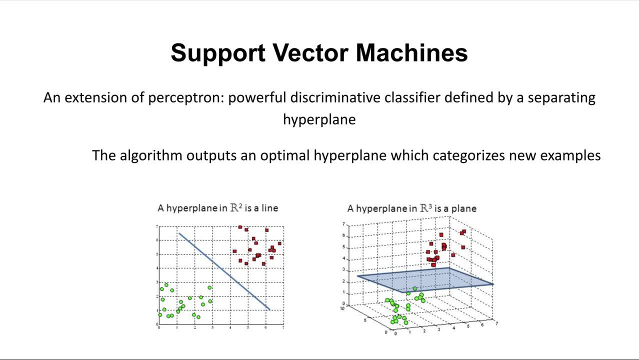 points. Each example or data point you see in these graphs is known as a support vector, thus the name of the algorithm: support vector machines. And this is possible for multi-dimensional problems as well. right In two-dimensional spaces, hyperplane is a line. 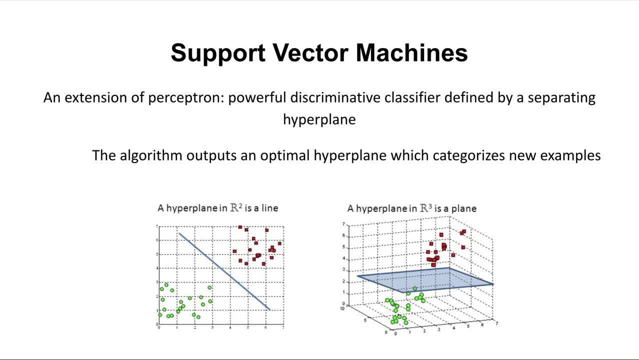 dividing a plane in two parts, where in each class lay in either side right, In R3, the third dimension, we have a multi-dimensional hyperplane, a hyperplane in vector space, actually a plane, and this divides between two data clusters and three. 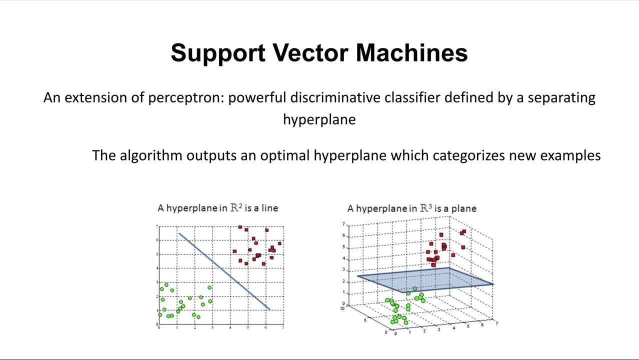 dimensions, and so that's really easy to understand. So the hyperplane is really just a fancy word for a line that is able to help us discriminate between two clusters of data, and that's what a support vector machine is defined by. A support vector machine is defined by its separating hyperplane, and that's why. 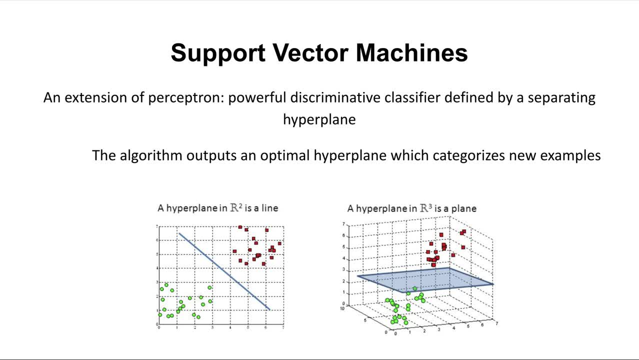 it is a discriminative classifier because the hyperplane is what the algorithm outputs and that helps us to discriminate between data clusters and also categorize new examples or new support vectors. So that's where we get the name Support Vector Machines and that's where the hyperplane is the most. 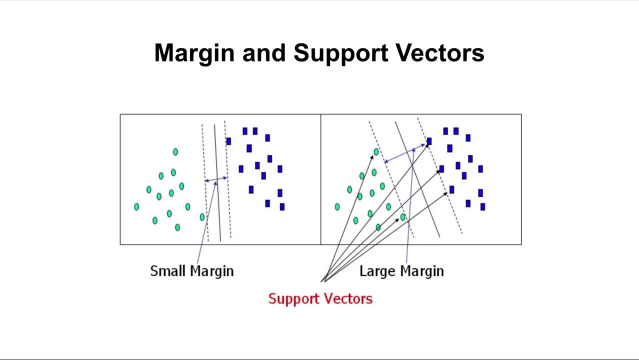 crucial part of a support vector machine. So let's break down some more vocabulary in support vector machines. So we've already talked about support vectors, right, or the individual data points- It can be of any dimension- that are involved in a support vector machine right in the algorithm. So it's another. 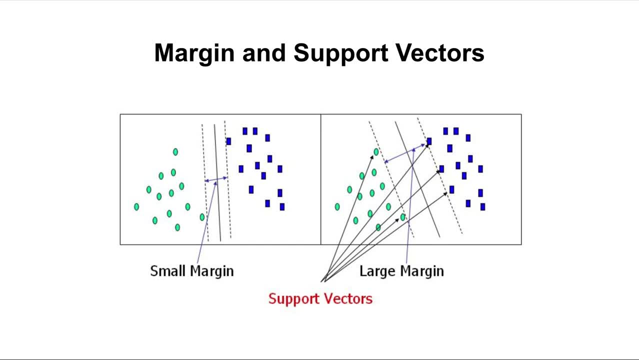 term known as the margin right. so in this graph I think it demonstrates what the concept of margin really well. and graph one: on the left you see that margin is basically the size of that hyperplane on both sides. right It's the 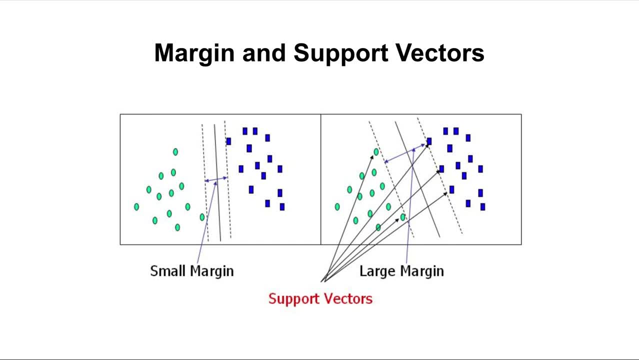 length of the hyperplane from each consecutive data point, from the nearest data point, And so a hyperplane with a really small margin is relatively close to both data clusters on both sides. A hyperplane with a large margin has really far distance from both data clusters on both. 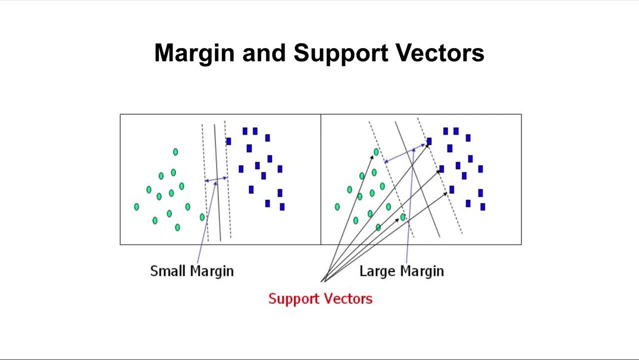 sides And that's important to know, because now you can talk about hyperplane having small or large margin, And when we get to how to tune support vector machines and understanding hyperplanes in more complex dimensions, margin is a really important concept, because margin really 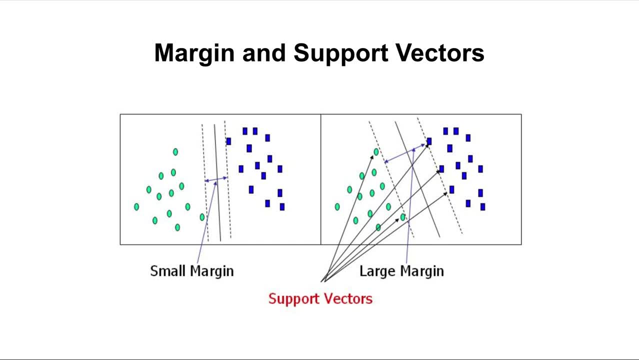 is what we think about when we think of minimizing loss for our support vector machine. So understanding the concept of small margin being very close to the data point clusters and large margin being very far from the data point clusters is huge to understand. And once again, just to reiterate from the last slide, support vectors are really just 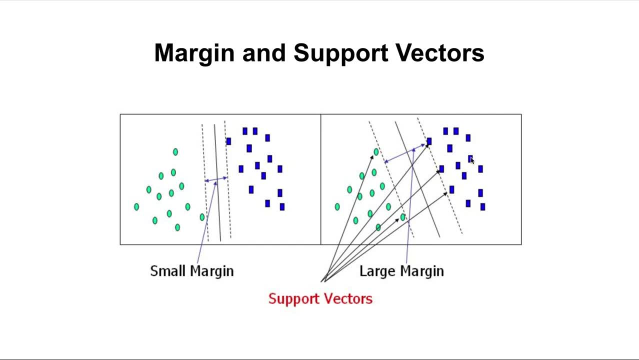 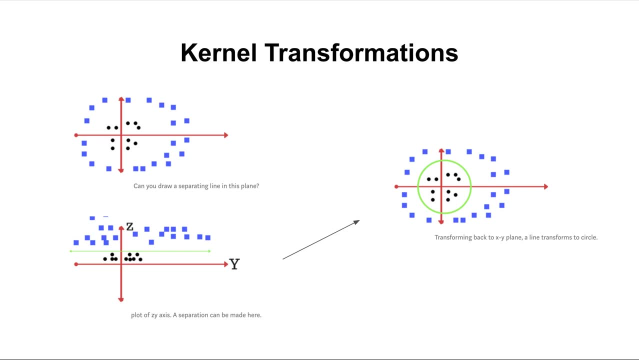 those individual data points that fall in the tumultuous space of the model, right? Let's move on. Let's talk about something that seems really complex, right? But I'm going to break this down and make it really easy for you to understand. So, if you take a course in linear algebra or any, 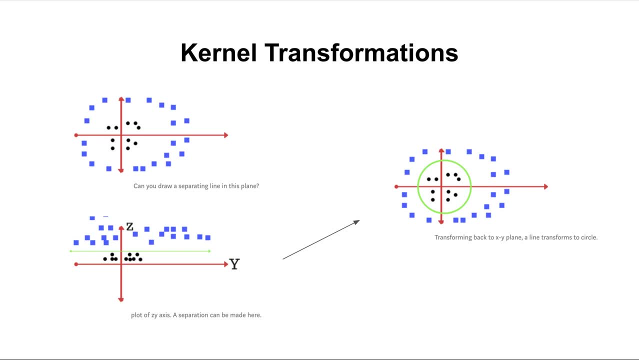 kind of matrix-based or vector-based class. then you probably have heard of transformations for vectors or matrices, right? A matrix, in essence, is a transformation of some dimensional space, right? And so let's talk about this problem. So, in the topmost graph, 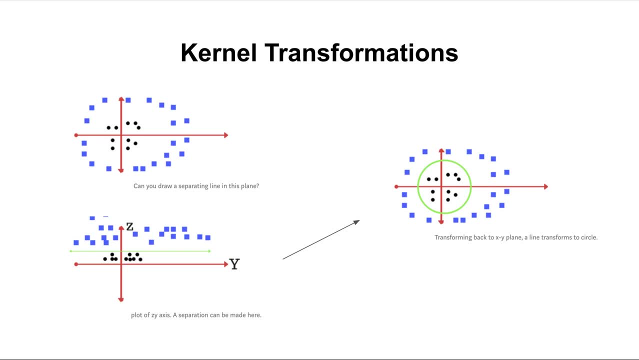 the graph, in the top left, my top left corner, you see two clusters of data points. You have blue data points on the outside- that forms a separate circle, and you have the red or black data points that form a smaller circle on the inside. And the question is: can you draw a? 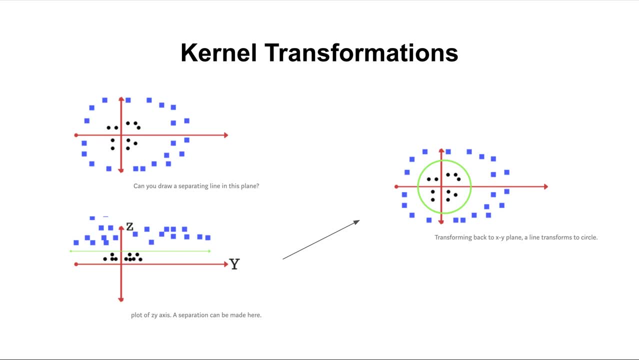 separating line in this plane. This is a very interesting question because, as I said earlier, these data clusters are made to be circular. So if you have a data cluster that's made to be circular, then you can't draw a separating line. So when you think about how to draw a separating 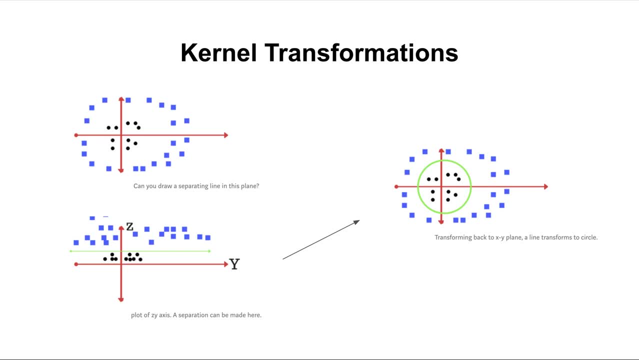 line. you can't really draw a separating line because these are circular data clusters and you can't really draw a line to describe something that's in a circular formation, right? So that's not possible. So we are applying something known as a kernel transformation to this data. The graph: 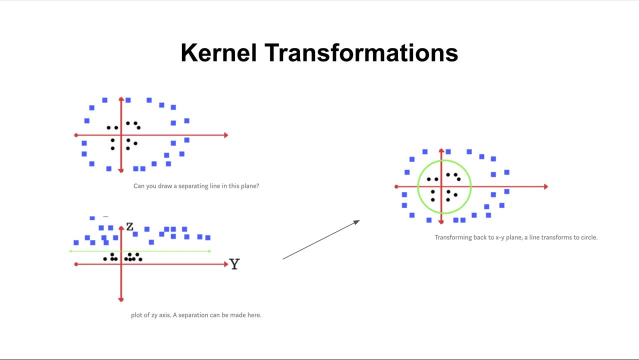 right below that, the y versus z graph. we've transformed this data to represent it in a different dimensional space. This is a plot of the z graph and we're going to draw a separating line on the y-axis, and now we can actually make a separation, which is really cool. And there we go. 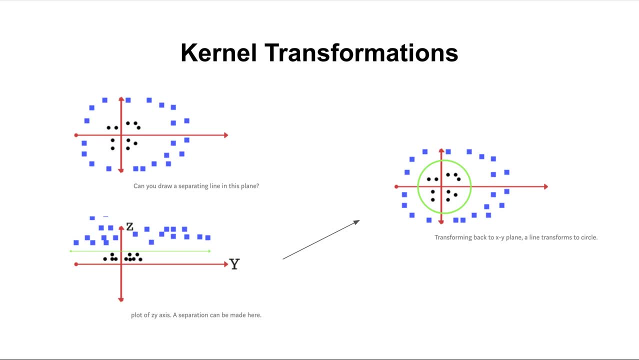 We made a really nice separating hyperplane line and that's awesome. So that process of going from that circular clustered graph to changing the dimensions of the graph right, changing the size, the dimensionality of the graph- is known as a kernel transformation And it's really important. 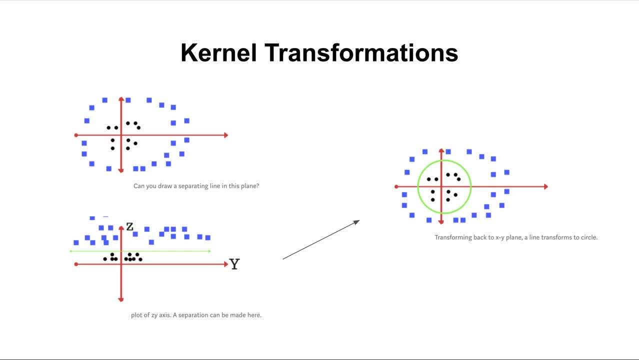 to understand these because, especially in the next video, when we talk about principal component analysis and dimensionality reduction, kernel transformations are a huge part of machine learning. because kernel transformations are essential to have support vector machines. It's essential to have these kernel transformations right Because in these kernel transformations we're basically 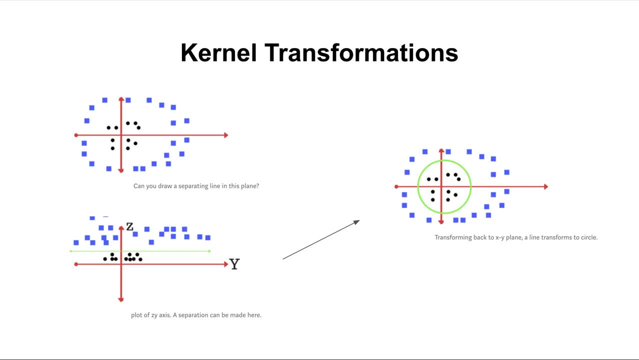 transforming a line in the original plane and we're mapping it to some more difficult environment, right. So to make that easier to understand. we have a really complex circular data environment in the first graph And after we transform it with the kernel transformation, we basically transform. 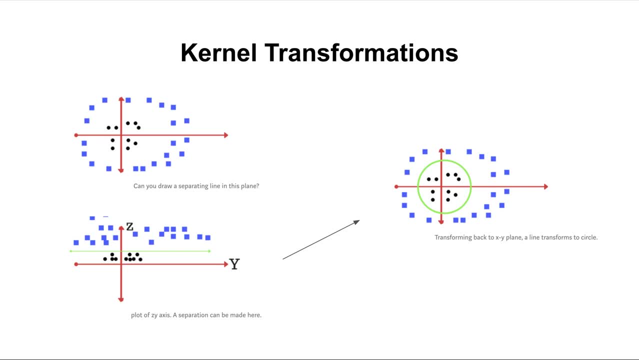 it into a dimension or a set of dimensions where it's easier to visualize and easier to draw a separating hyperplane. And that's the essence of kernel transformations: We're basically taking something difficult to divide to make it something that's easy to divide, And then we can also 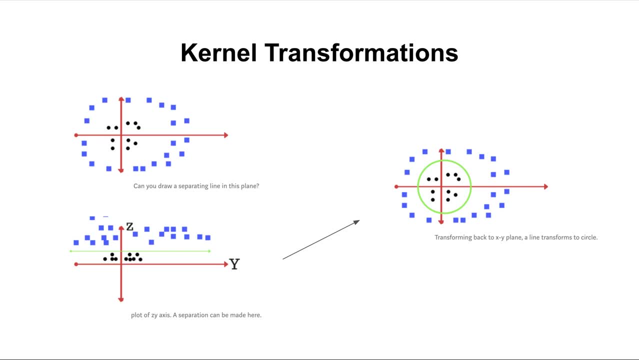 actually visualize this as a circle right? If you go back to the original xy plane, you could technically draw a separating hyperplane in the form of a circle right? But that's definitely more complex, right? And the idea is that when you implement support vector machines in Python with Scikit-learn, you don't. 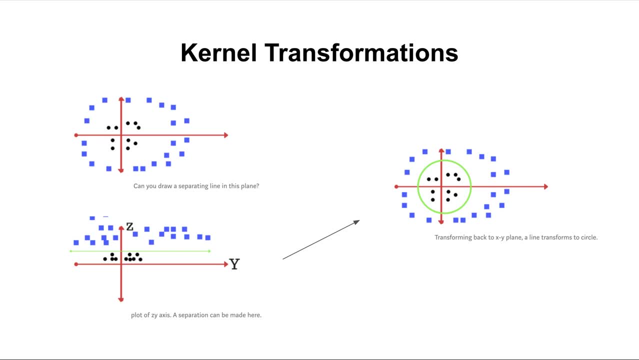 have to actually guess or derive the transformation every time for your data set right, And typically transformations will be much harder than these ones, And the idea is that the Scikit-learn library for Python SVM's implementation provides it inbuilt right. You don't ever have to guess or derive the. 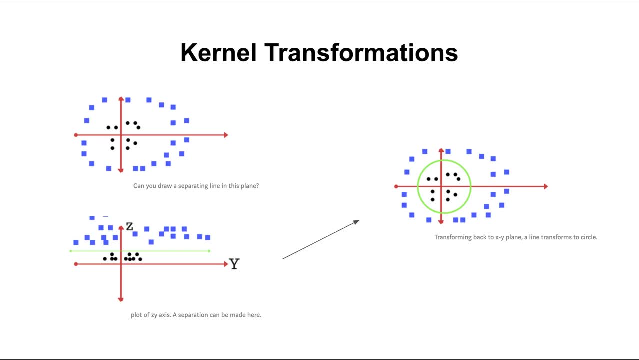 transformation And kernel transformations are super useful, right? Because, as you can see, the little algebraic dimensional manipulation, you're able to reduce this problem to a much more easier scenario, And that's why kernel transformation is super important across all machine learning, not just support vector machines. And let's move on. So I talked about the cost. 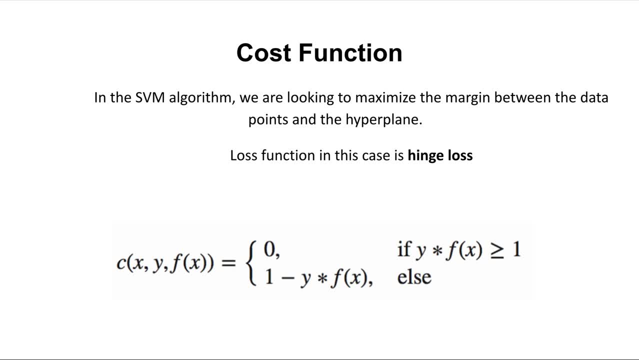 function for logistic regression. Let's break it down for support vector machines. In the support vector machine algorithm we're looking to maximize the margin between the data points in the hyperplane. In this case, the loss function is known as the function of hinge loss. You don't really have 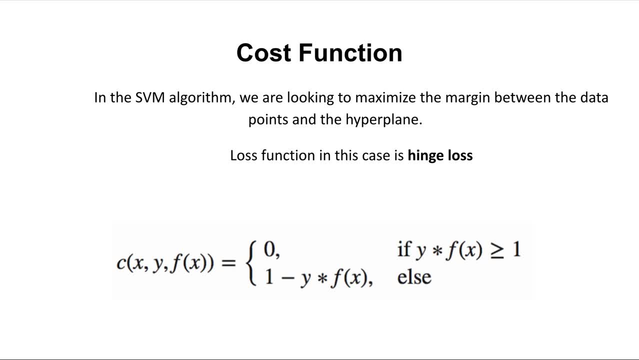 to understand the mathematics behind this, because this is definitely out of the content covered in this lecture series. But the idea is that you're not going to have to use the same loss function that you use for logistic regression or linear regression, And it's a completely different maximization problem. 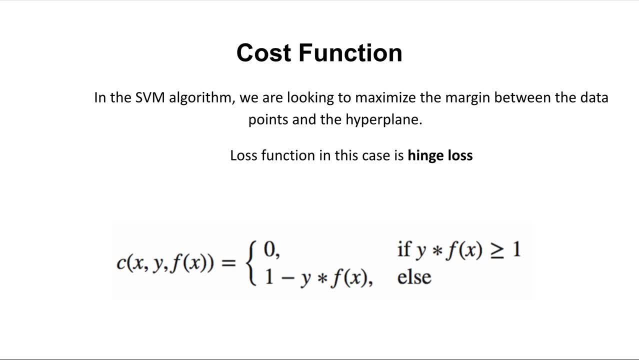 Instead of trying to maximize the accuracy of the model in terms of reducing the loss function, you're trying to maximize the accuracy in terms of maximizing the margin between the data points in the hyperplane. So that's the broad thing I want you to understand on this slide. It's that for the 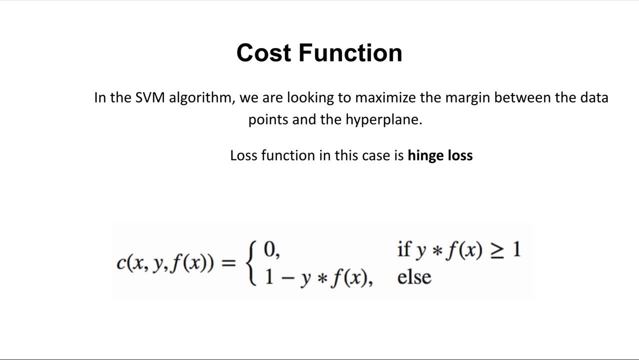 cost function in an SVM algorithm or for when we were trying to reduce the loss, to reduce the loss in a support vector machine. we're basically looking to maximize the margin between the data points in the hyperplane. So think about that. A bigger margin is better in terms of minimizing our. 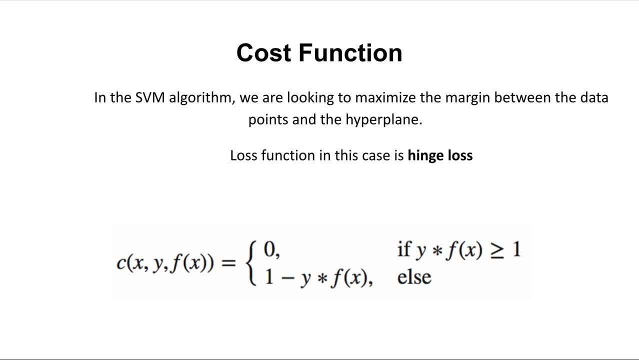 loss And the actual loss function is known as the hinge loss function, And I'm not going to explain the mathematics right now because it's definitely difficult to understand. So you can look into that yourself And I guess we'll continue. Let's talk about tuning of support vector machines as one of 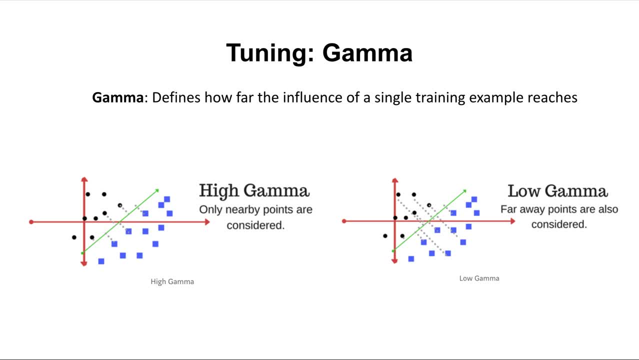 the last topics for today. When we tune a support vector machine, there's a parameter known as the gamma. The gamma is an important parameter because it defines how far the influence of a single training example reaches. There's high gamma support vector machines and there's low gamma. 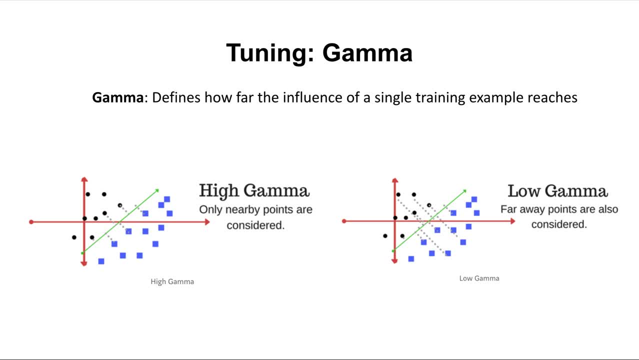 support vector machines. Let's take a look at the high gamma support vector machine example. In a high gamma support vector machine, only nearby points are considered And that comes back to the original definition right. The gamma parameter defines how far the influence of a single training example. 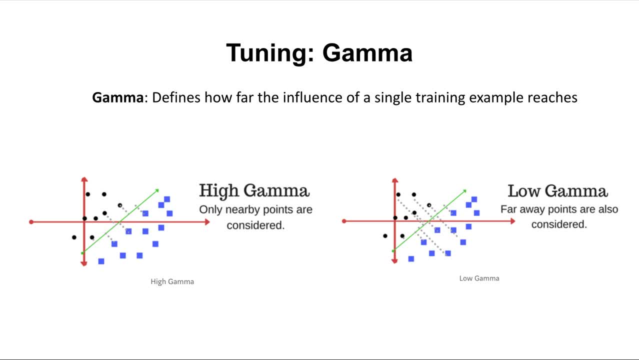 reaches. So that means that in a high gamma example, only nearby points will be considered, right, Because we're giving very little influence to the single training example, right? So we're only considering nearby points. So if we had some crazy outlier, that wouldn't be considered at all. So 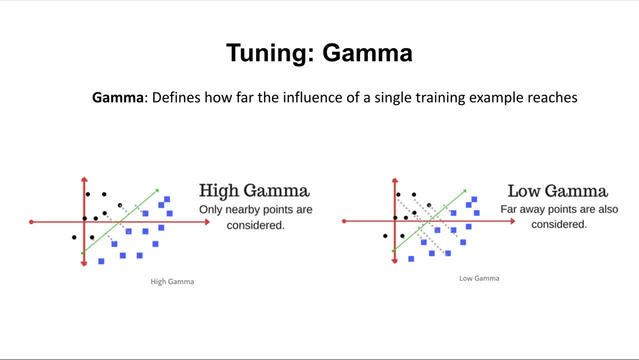 we'd have very high gamma And that wouldn't affect the influence of the nearby training examples. So what I'm trying to tell you is this: The higher the gamma, the more local we stay in our support vector machine. In other words, the more nearby points we consider when we're high gamma. When we're low gamma, we 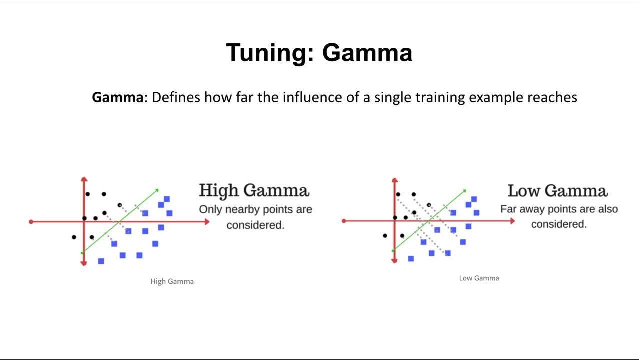 also consider far away points that may not be as easy to describe for a support vector machine right And the far away points could be like outliers: They could be really distant. They could be pretty decently far from the hyperplane. So it's important to understand high gamma versus. 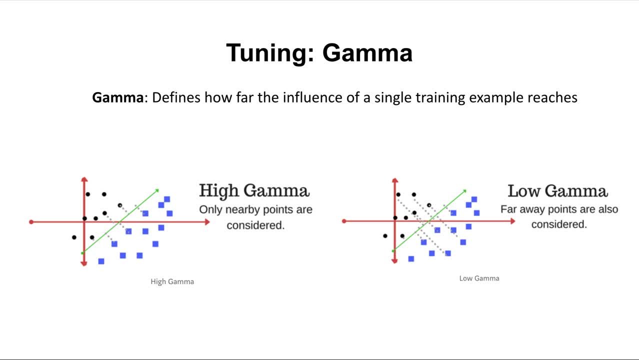 low gamma. So for training purposes, this is one of the parameters that we adjust in our support vector machine when we try to maximize the hyperplane right To reduce loss, And so it's really important to understand that gamma is a really important hyperparameter that we adjust constantly in our tuning of the model. 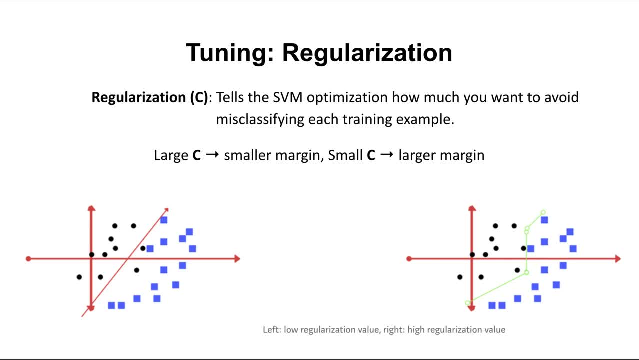 Another tuning parameter is regularization parameter, or C, defined as C. This is a parameter that tells the support vector- machine optimization- how much. you want to avoid misclassifying each training example, Let's break that down. Let's take a look at those two graphs. 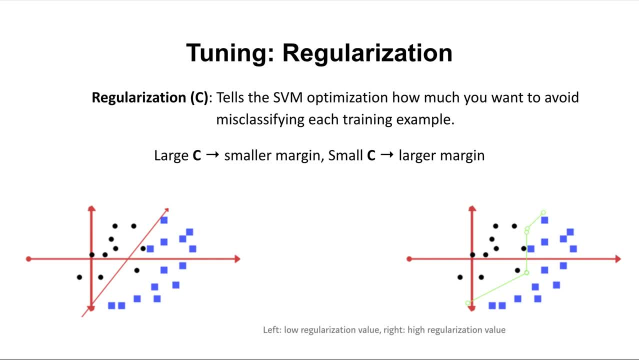 On the left we have a low regularization value graph and on the right, we have a high regularization value graph. On the left, you basically see a graph with a really simple line. right, It's basically just drawing one training line, one hyperplane, and it's being very broad. right, It's just basically saying let's divide this as best as we can without complicating our hyperplane too much. right, And it actually does actually make some oopsies. right, You can see that there's two data points that fall on the wrong side of the hyperplane. right, The two black circles. That's bad, right. 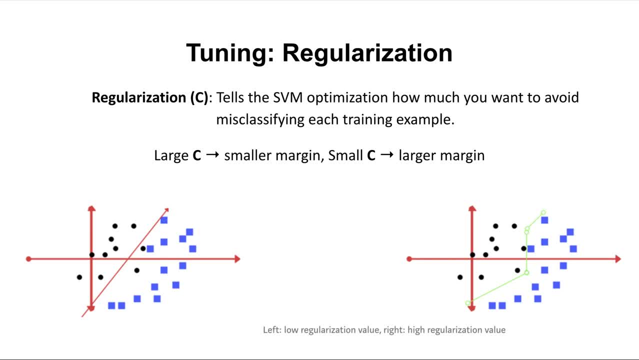 Right. But sometimes that's not a bad thing necessarily for the accuracy of our model, because sometimes you may want to prioritize overall accuracy of the support vector machine over the misclassification of a few training examples. right, Like the two black points, And then you have a high regularization graph on the right. This time we have a much more different support vector machine hyperplane. This is a much more complicated support vector machine hyperplane because in this case we're actually making a bunch of twists and turns right. 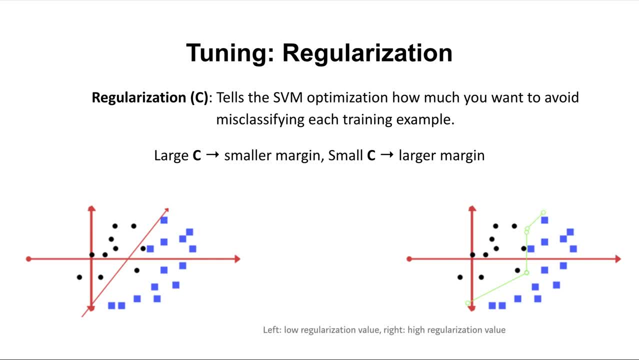 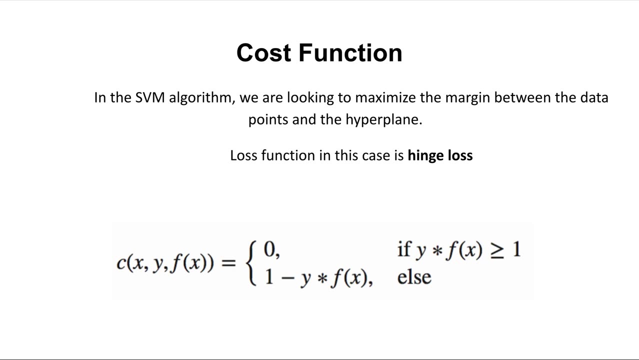 So it's actually nice in the sense that we're actually classifying all of our examples correctly, but this comes at the cost of a very different hyperplane, a very much more difficult to optimize hyperplane, because, think about it, When we talk about the cost function for support vector machines, it all comes down to maximizing the margin between data points in the hyperplane. 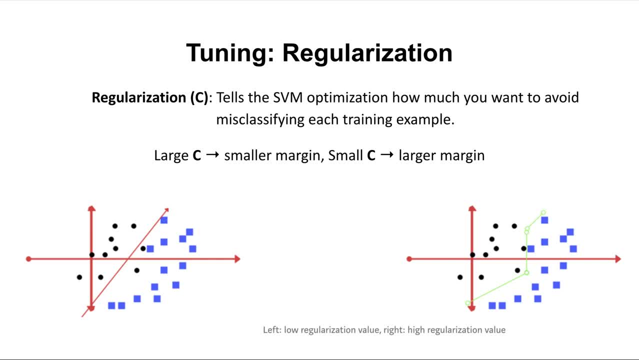 In this case, with very small, very large, high regularization value, it's actually very difficult to maximize the size of the hyperplane, which is a bad thing, right? So remember, it's a trade-off. This is all a trade-off, right. 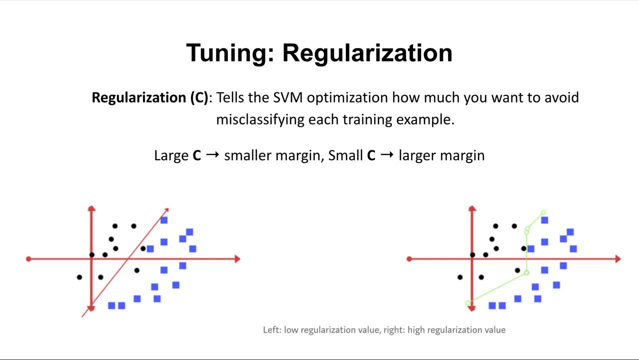 You're trying to basically get that. It's a trade-off between the overall accuracy of the model, the support vector machine, and whether you're misclassifying a few data points or support vector examples, right? So remember, machine learning, hyperplanar tuning, is always a trade-off, right. 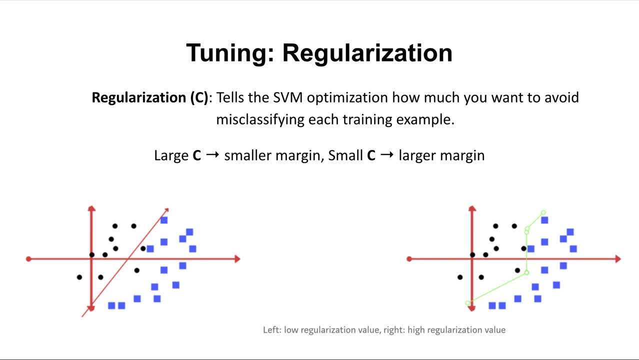 Going back to when we talked about linear regression with a learning rate. right, If you increase your learning rate by a lot, you get there faster. right, You prioritize speed, But you have the issue that you might overshoot your lower loss minimum point on the parabola of loss, right. 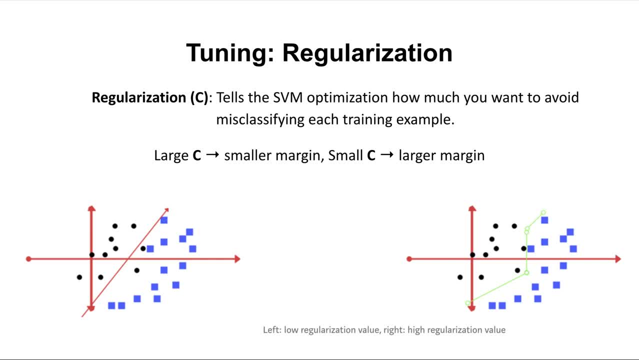 Which is bad. But if you have a really small learning rate, you're definitely going to hit the point exactly where you want it right. You're definitely going to hit the loss minimum. But it just takes practice. It takes forever. So remember, it's always about finding that hidden perfect balance where you get the best of both sides in the trade-off. 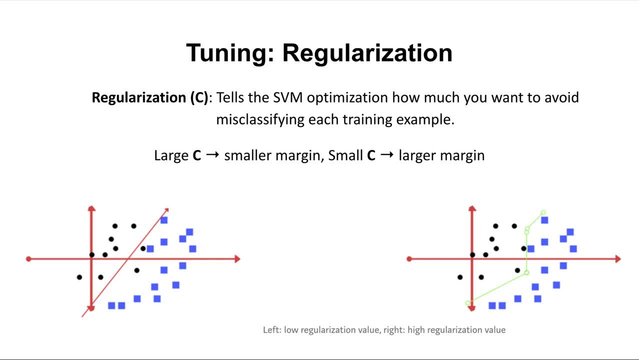 That's what tuning is all about, right, And I guess for regularization it's the same thing, right. Do you want that perfect, completely accurate model, but with a really bad hyperplane with high loss? Or do you want a broad hyperplane that actually has higher accuracy overall, but it does misclassify? a few examples. 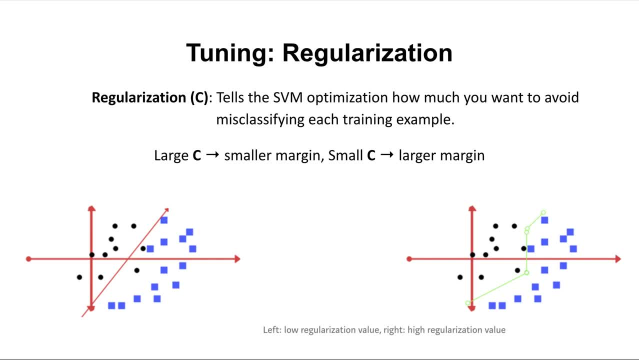 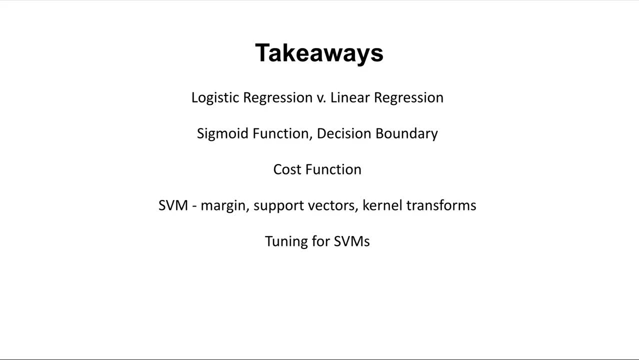 It's really just a push and pull and an overall trade-off, And even in the model you have to try to balance those two interests very carefully. So that's it for today, But let's conclude the lecture. The takeaways for today's lecture is that we talked about logistic regression versus linear regression. 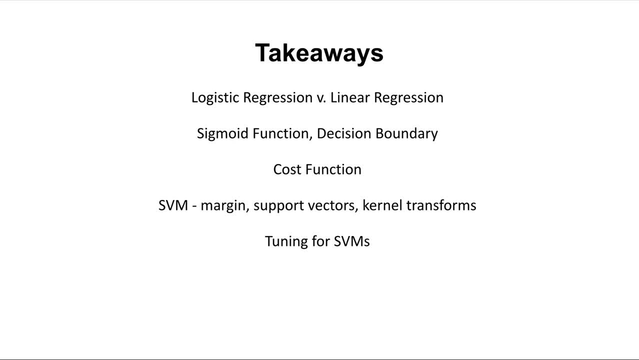 The idea of the decision boundary, the sigmoid function, etc. We talked about the cost function for both logistic and SVM, And for logistic regression we talked about how the cost function is cross entropy right Instead of linear regressions mean squared error. 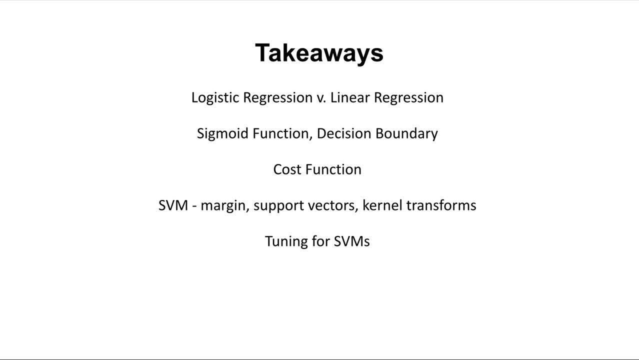 And then for support vector machine. For support vector machine, our cost function is hinge loss And for support vector machines we talked about margins, support vectors, kernel transforms, how to tune them with the gamma and regularization, etc. And I just hope that today's video is really helpful for you to understand these more advanced classifiers right. 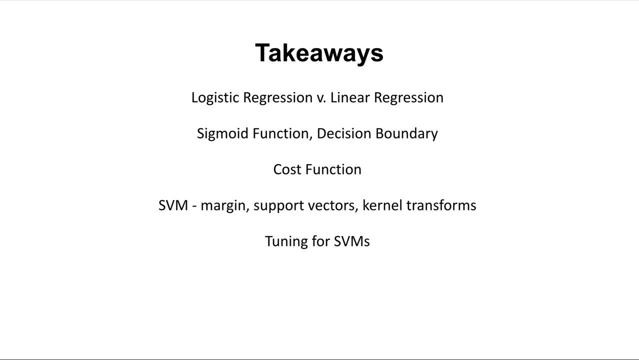 Because we talked about really simple classifiers like a decision tree last time, But today's examples were much more heavyweight classifiers, right Ones that are used in academia and industry much more often, And these classifiers are not as easy to understand. So I hope that today's video was helpful.